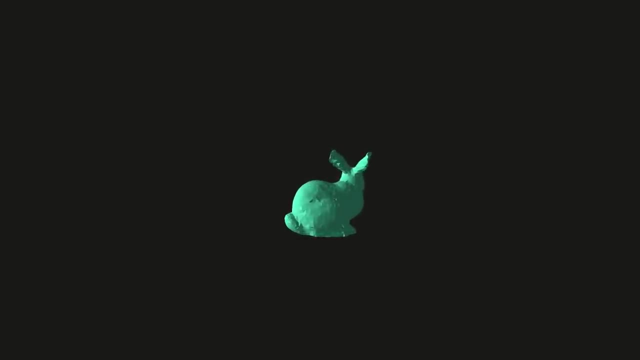 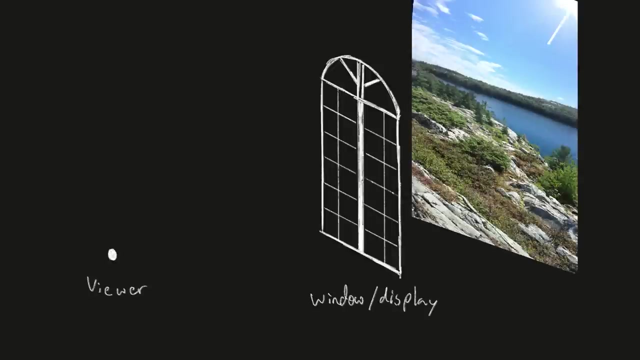 them out of many triangles. To create an accurate 2D representation, we need to project each of these triangles onto a flat plane. from the perspective of a viewer, It can be helpful to think of a computer screen as a window where light bounces off of an object through. 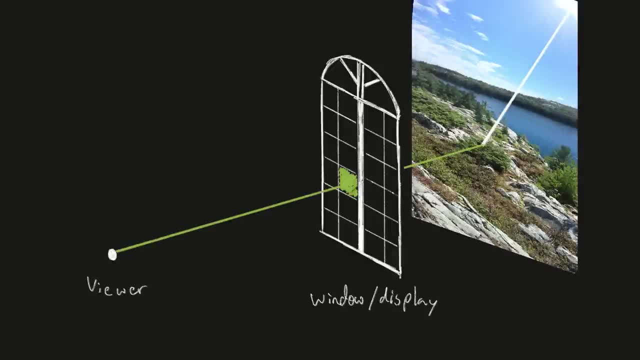 the window and into your eye, So to generate an image. it's almost as if we need to do the reverse operation. If you shot a ray from your eye through each section of the window, what colour would you hit? And this is the basic idea behind 3D graphics. Each pixel of the display is like. 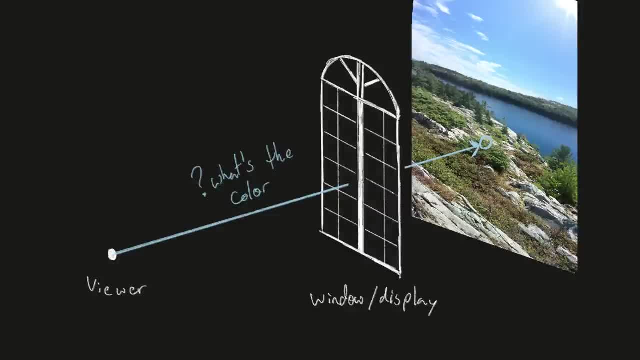 a little window and the more pixels, the clearer the image, And it is up to our graphics engine to figure out what colour of light would be passing through that pixel, as if the game world actually existed on the other side The method I've explained where rays are. 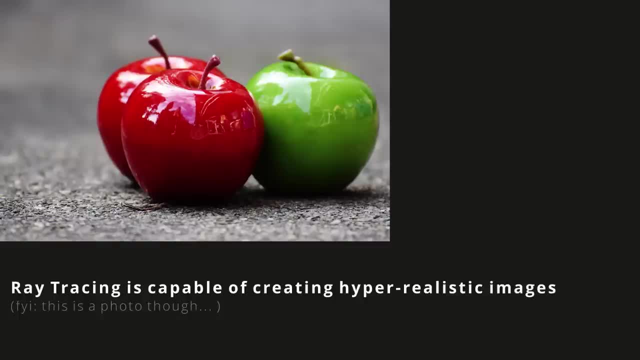 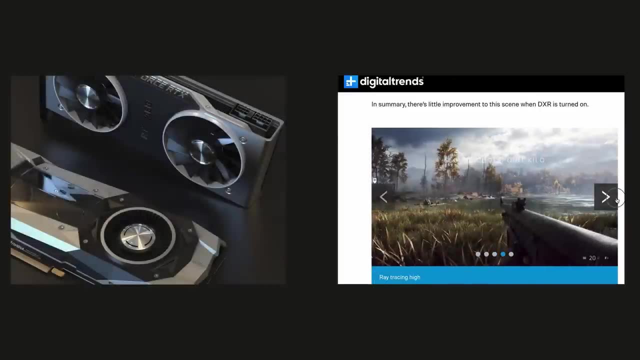 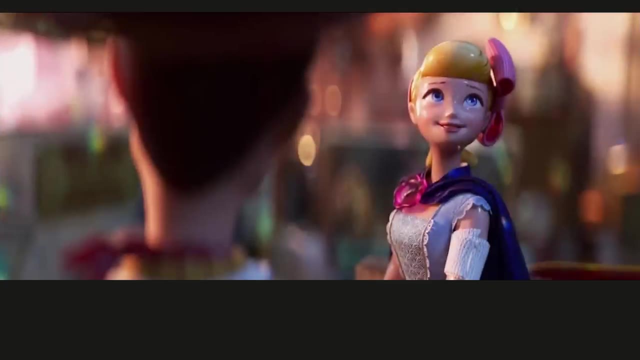 projected into the world and collide with objects is the foundation behind ray tracing. Ray tracing has only recently made its debut into video games, with the release of newer graphics cards containing dedicated ray tracing hardware. On the other hand, CPU-based ray tracing has been around for a long time and has been used extensively within the movie. 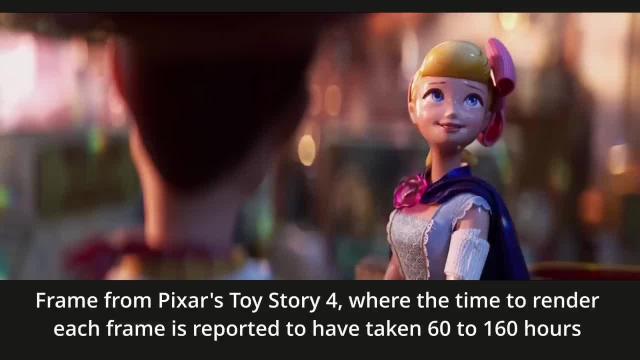 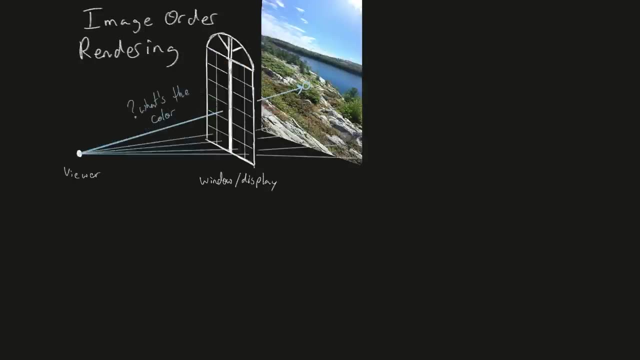 and animation industries, but it is much too slow to be used in real-time applications. Ray tracing in Toy Story 4 could take anywhere between 60 to 160 hours to render using CPU-based ray tracing. Ray tracing is known as image order rendering, since each pixel is first considered and 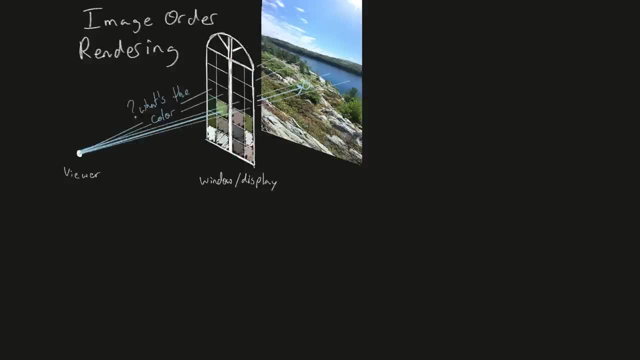 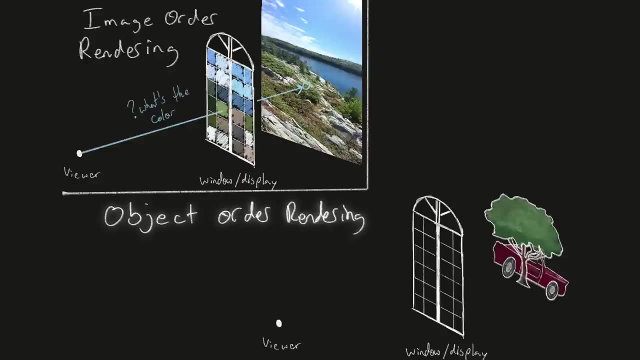 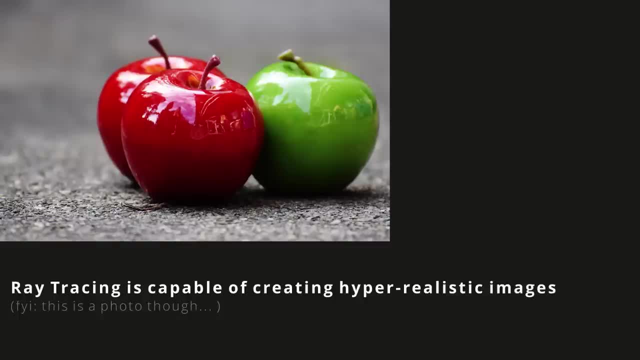 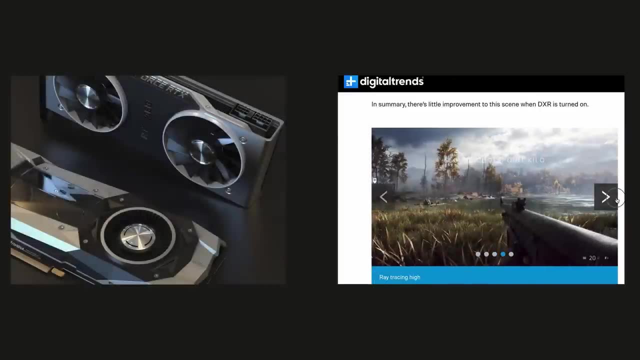 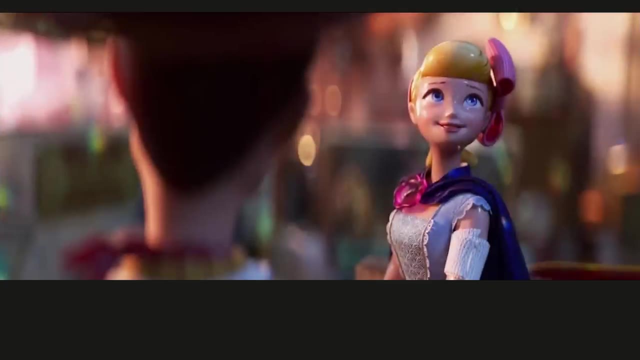 projected into the world and collide with objects is the foundation behind ray tracing. Ray tracing has only recently made its debut into video games, with the release of newer graphics cards containing dedicated ray tracing hardware. On the other hand, CPU-based ray tracing has been around for a long time and has been used extensively within the movie. 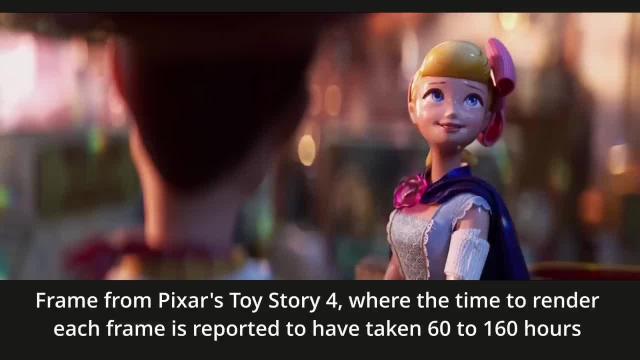 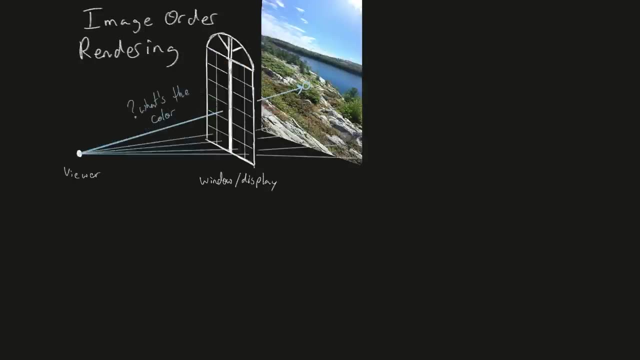 and animation industries, but it is much too slow to be used in real-time applications. Ray tracing in Toy Story 4 could take anywhere between 60 to 160 hours to render using CPU-based ray tracing. Ray tracing is known as image order rendering, since each pixel is first considered and 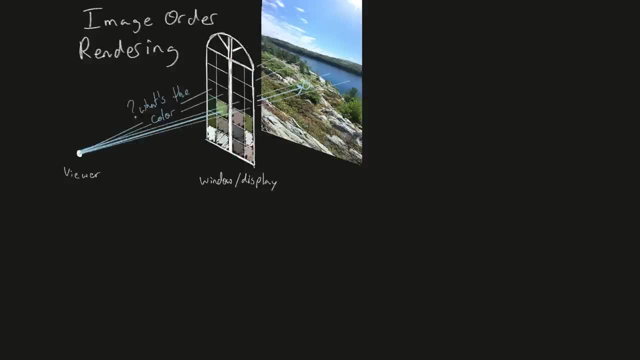 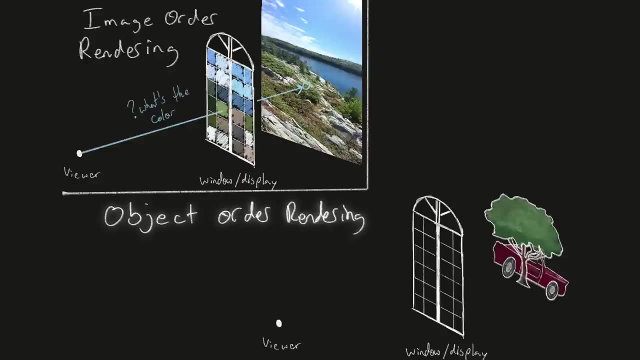 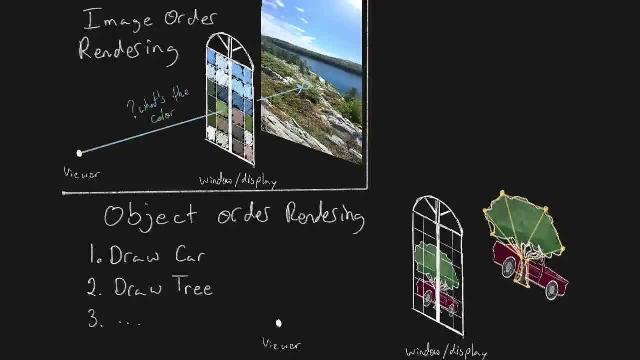 maps much better than the old way. This approach maps much better than the old way Since we can apply the same instructions but on different vertices in parallel. this way, we could find the location for each projected position within the vertex shader by calculating the line. 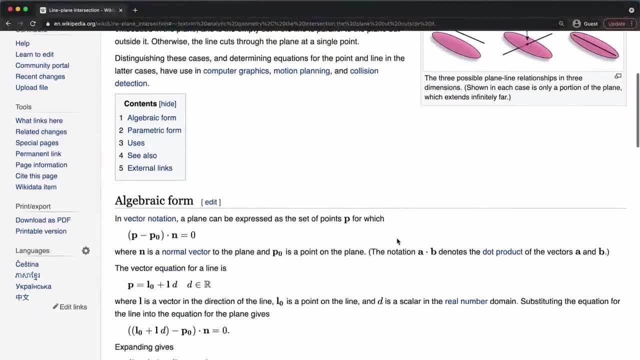 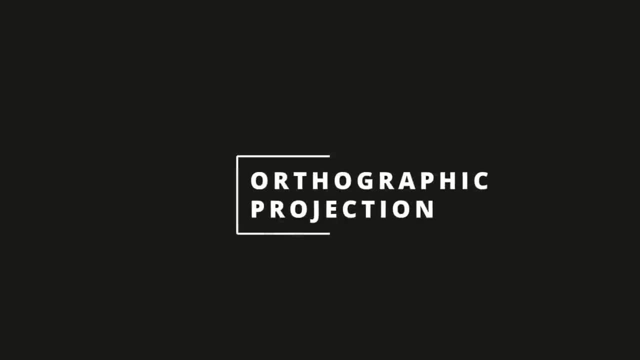 and plane intersection and this would work just fine. But a much more effective way to do this is with a matrix transformation. In the previous tutorial I talked about Vulkan's canonical viewings against other FreeD chairman features on helpful modo desk, because I find 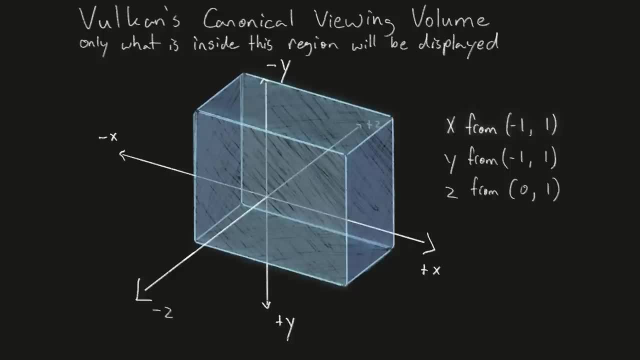 volume. Only the objects that are within this 2 by 2 by 1 region will be displayed. Note that the positive y-axis points down and positive z-axis points into the screen. An orthographic projection is a generalization of the view volume that allows us to specify whatever dimensions and whatever. 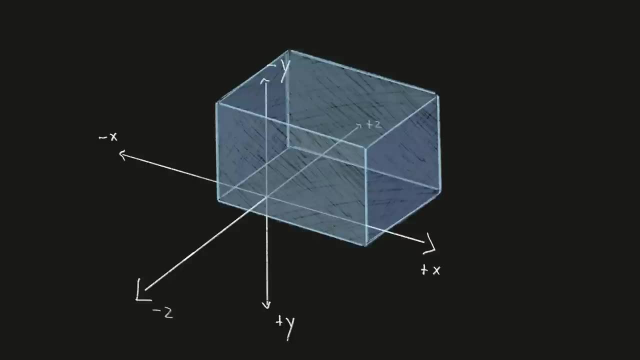 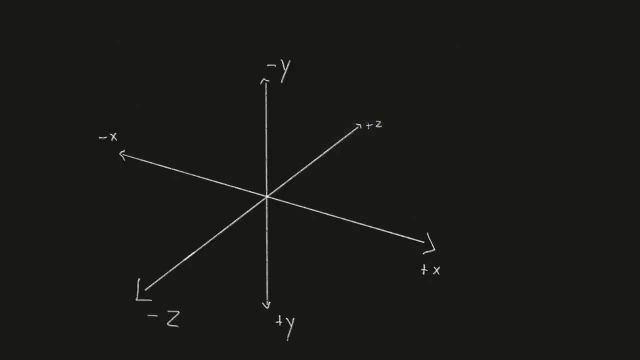 location we want but maintains the overall shape of the view volume and keeps the view direction and orientation fixed. The orthographic view volume is defined by six bounding planes: The left and right along the x-axis, the top and bottom along the y-axis and the near and far planes. 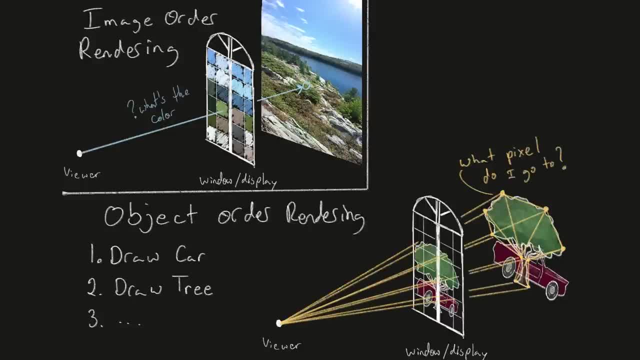 location for each projected position within a vertex shader by calculating the line and plane intersection, and this would work just fine. regionsphp version. to get that in a íre: in a vertex shader And using this option you should be able to see the exact. 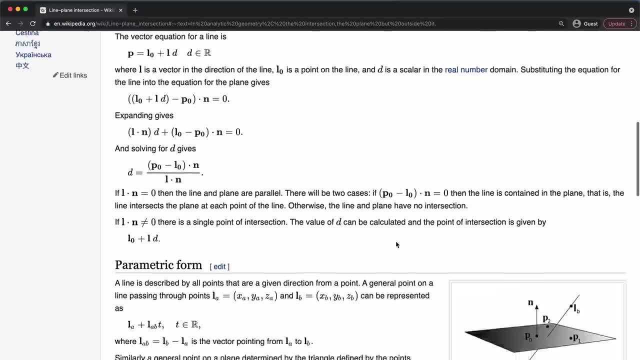 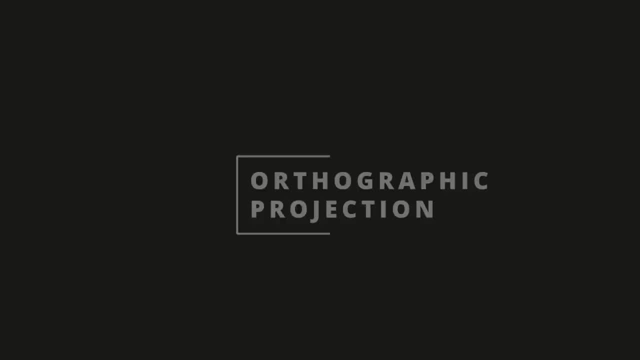 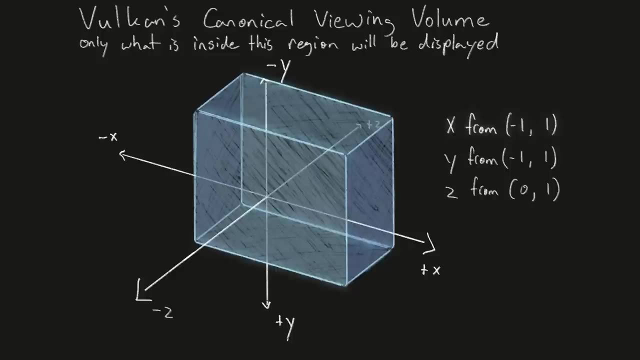 just fine, but a much more effective way to do this is with a matrix transformation. First, though, I want to start by explaining orthographic projection. In the previous tutorial, I talked about Vulkan's canonical viewing volume. Only the objects that are within this 2x2x1 region will be displayed. 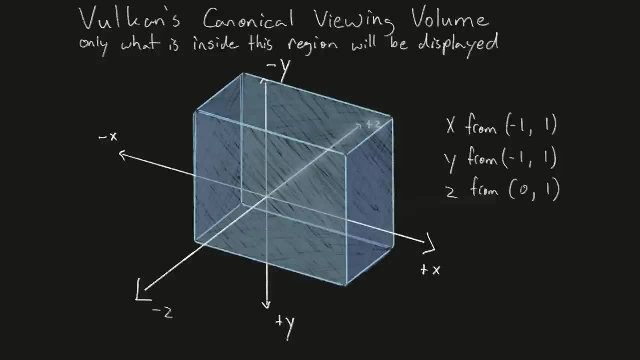 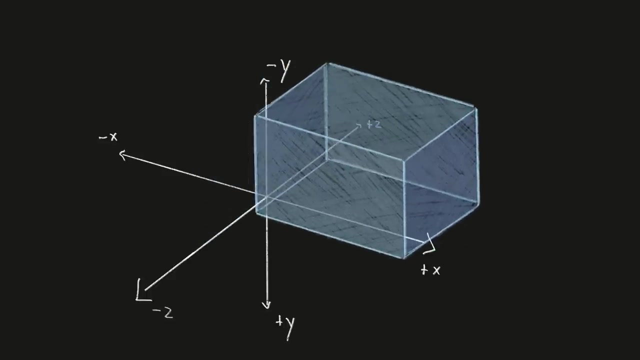 Note that the positive y-axis points down and positive z-axis points into the screen. An orthographic projection is a generalization of the view volume that allows us to specify whatever dimensions and whatever location we want, but maintains the overall shape of the view volume and keeps the view direction and orientation fixed. 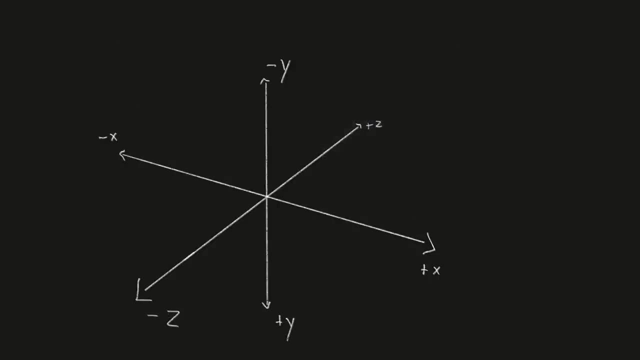 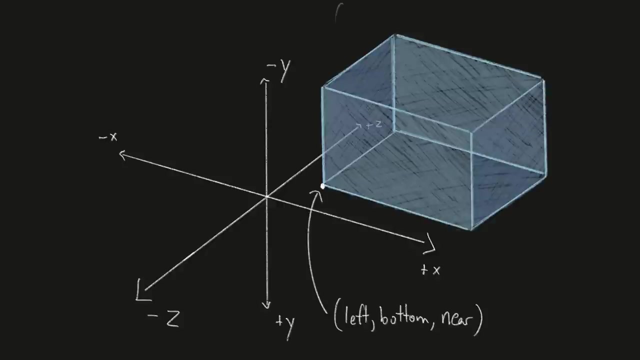 The orthographic view volume is defined by six bounding planes: The left and right along the x-axis, the top and bottom along the y-axis and the near and far planes along the z-axis. So these six values- left, bottom, near and right, top, far- define the orthographic viewing volume. 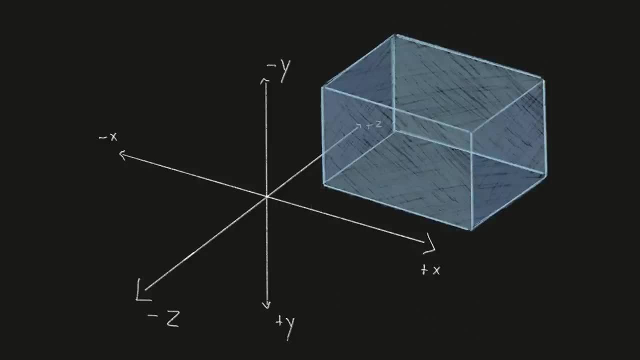 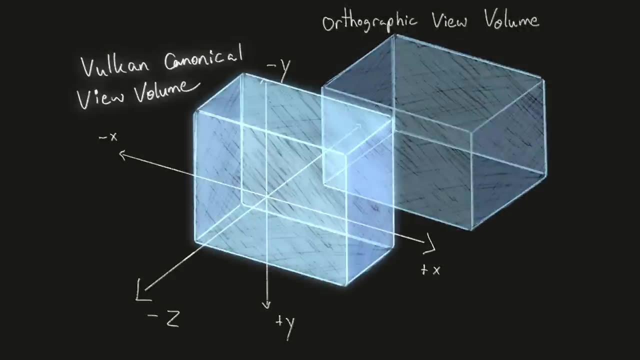 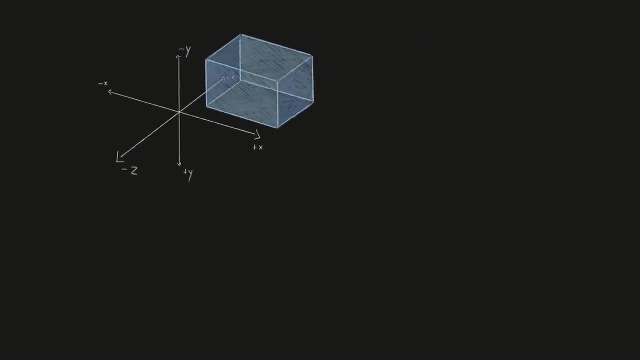 So to construct an orthographic projection matrix, we need to solve the following problem: How do you transform the orthographic view volume to Vulkan's canonical view volume? And the good news is we already know how to do this. We can combine two basic transformations. First, translate the box so that the center of the 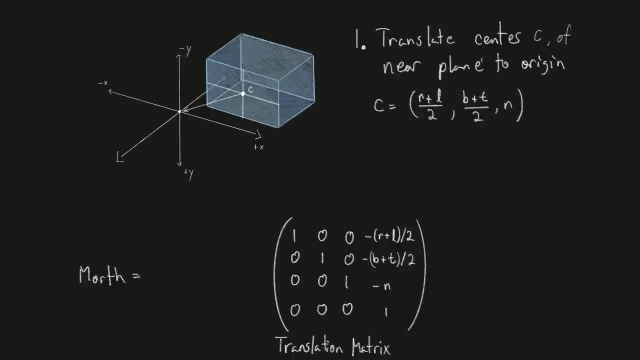 near plane is at the origin. Then follow that with a scale transformation so the boxes have the same dimensions. So the numerator will be the canonical view volume's dimensions and the denominator will be the dimensions of the orthographic view volume. If we multiply the matrices and simplify, we get the orthographic projection matrix. 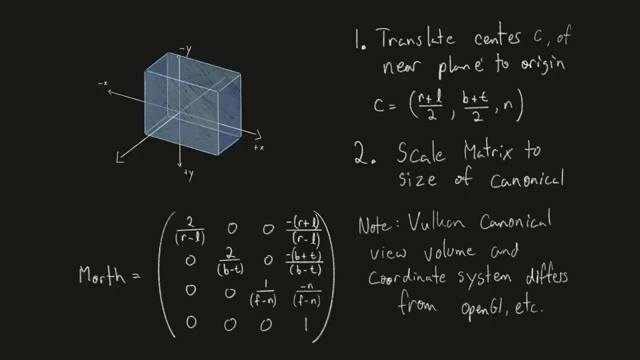 Note that this matrix differs slightly from most other online resources. The canonical open-gen open-gl view volume is a cube with a z-range of negative one to one. Additionally, open-gl uses a left-handed coordinate system and looks down the negative z-axis. 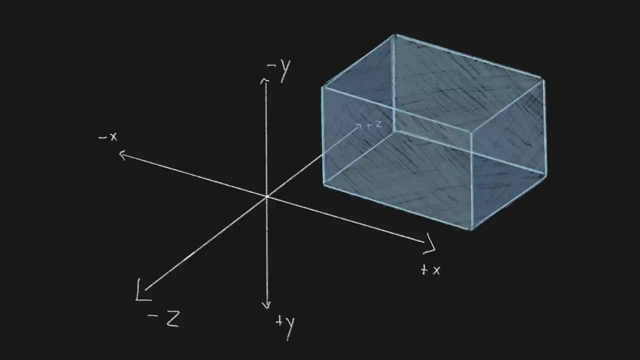 along the z-axis. So these six values- left, bottom near and right top far- define the orthographic viewing volume. So to construct an orthographic projection matrix we need to solve the following problem: How do you transform the orthographic view volume to Vulcan's canonical view volume? 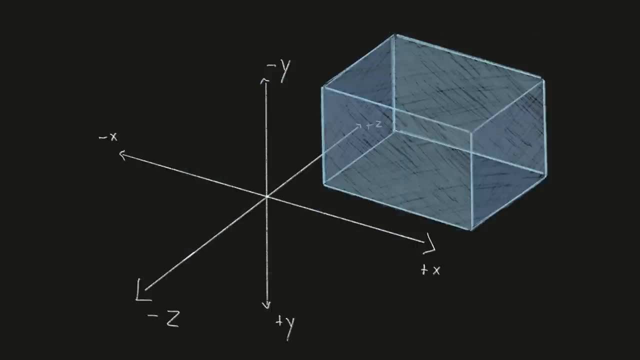 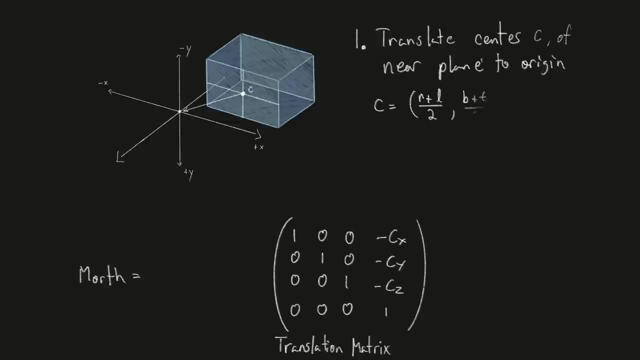 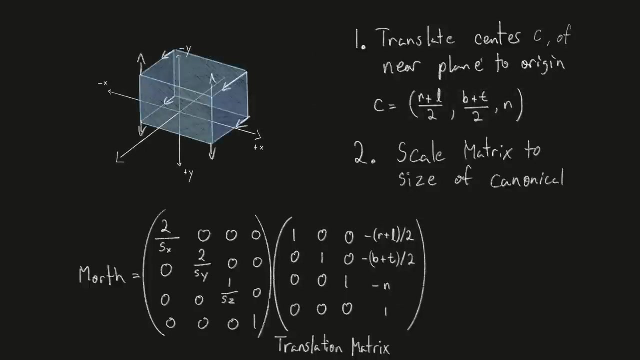 And the good news is we already know how to do this. We can combine two basic transformations: First, translate the box so that the center of the near plane is at the origin. Then follow that with a scale transformation so the boxes have the same dimensions. 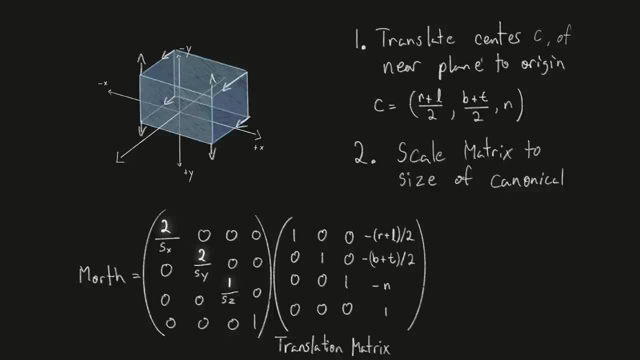 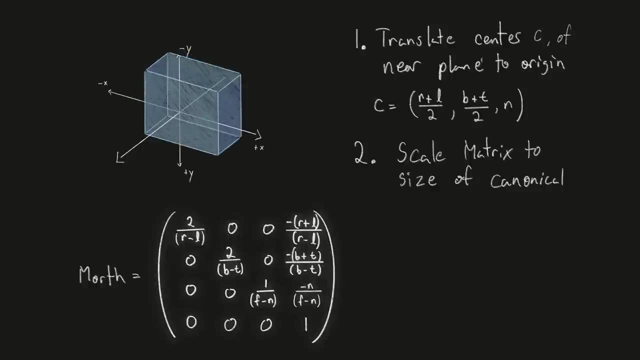 So the numerator will be the canonical view volume's dimensions and the denominator will be the horizontal view volume's dimensions. The denominator will be the canonical view volume's dimensions and the denominator will be the dimensions of the orthographic view volume. If we multiply the matrices and simplify, we get the orthographic projection matrix. 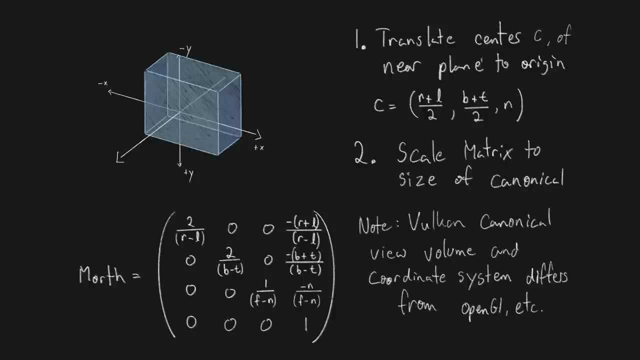 Note that this matrix differs slightly from most other online resources. The canonical OpenGL view volume is a cube with a z range of negative one to one. Additionally, OpenGL uses a left-handed coordinate system and looks down the negative z-axis, but we're using a right-handed coordinate system and looking down the positive z-axis. 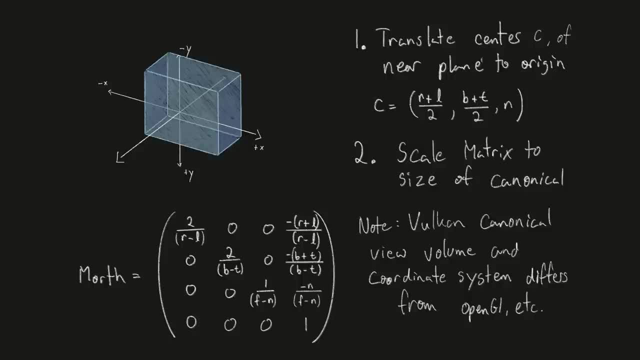 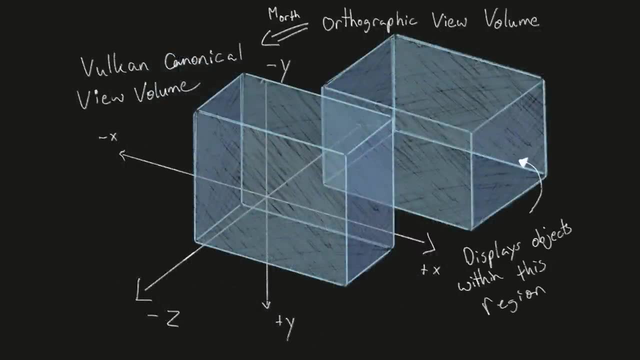 So just keep this in mind if you are following other resources with different conventions. And that's it. By applying this transformation to our objects, the objects that are within the region occupied by the orthographic view volume will be scaled and moved into the region covered by the canonical view volume. 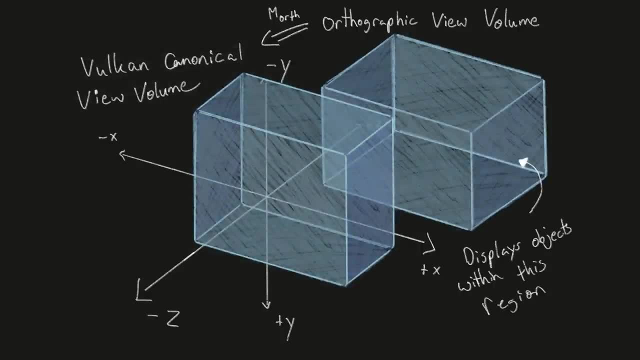 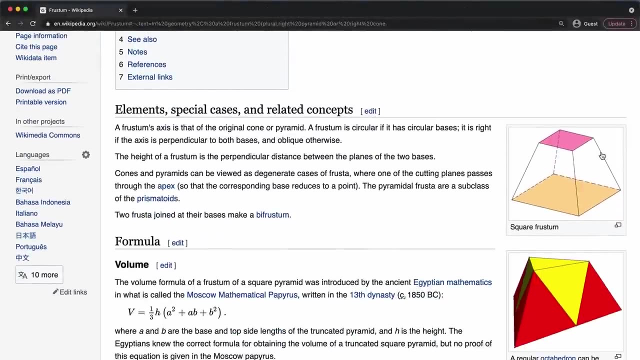 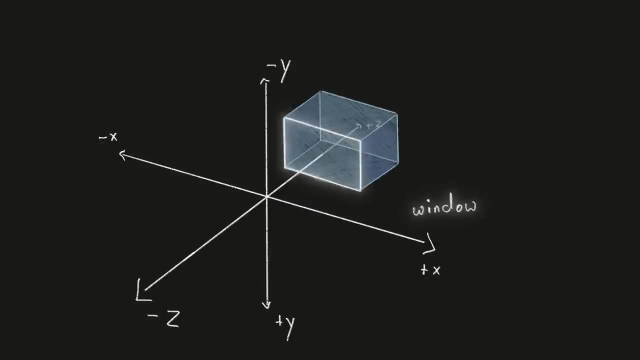 and therefore the objects will be displayed. But the orthographic view volume doesn't apply perspective. To do that, we require a viewing volume that is not box shaped, but a shape known as a square frustum. A frustum is the shape that captures a viewer's line of sight. 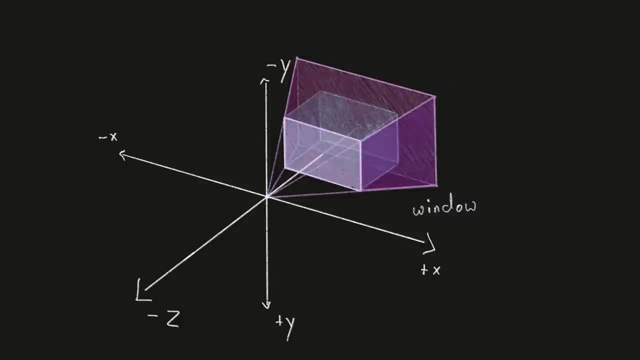 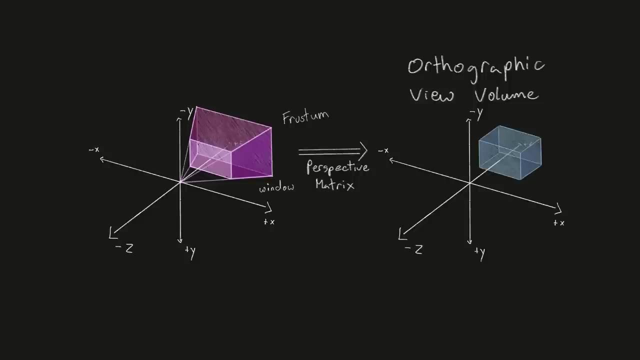 as if they were looking through a rectangular window. So what we want is a perspective matrix that transforms the frustum and any object it contains into the orthographic view volume. Doing so would apply perspective to all objects within this space. The farther away an object is, the smaller it will appear. 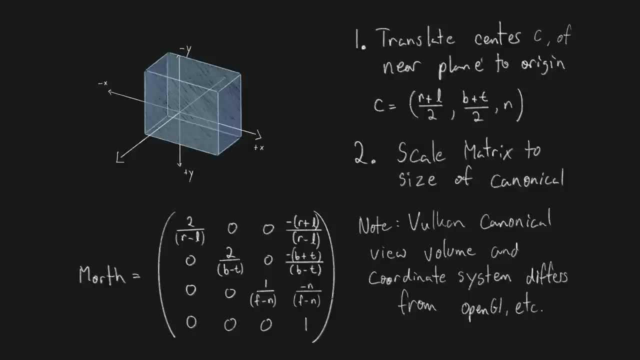 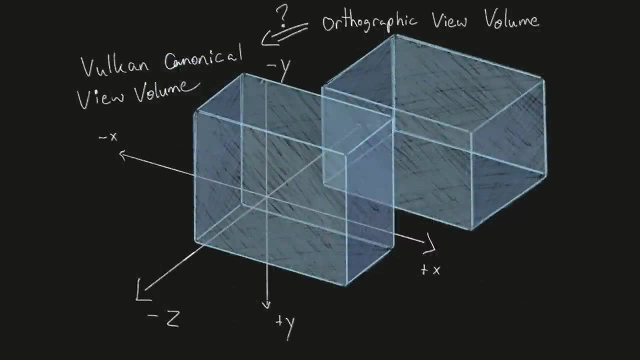 but we're using a right-handed coordinate system and looking down the positive z-axis, So just keep this in mind if you are following other resources with different conventions. And that's it. By applying this transformation to our objects, the objects that are within the region occupied by the orthographic view volume will be scaled and moved. 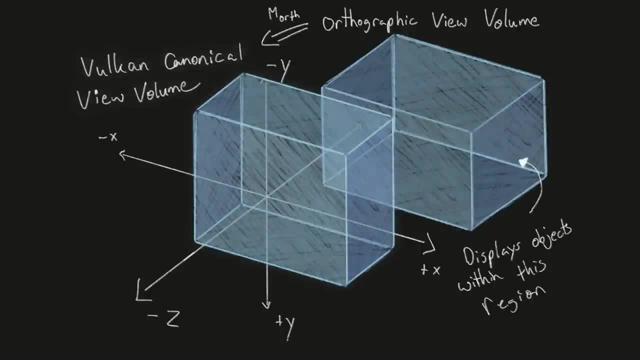 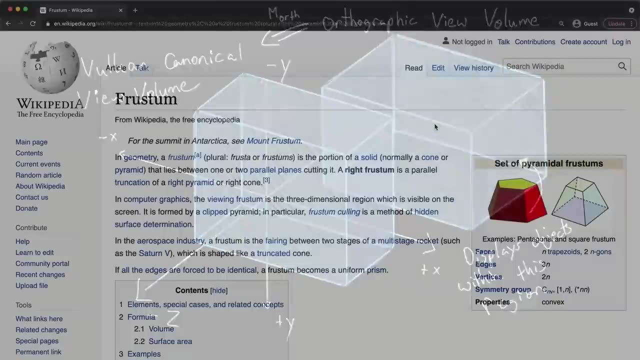 Into the region covered by the canonical view volume And therefore the objects will be displayed, But the orthographic view volume doesn't apply perspective. To do that we require a viewing volume that is not box shaped but a shape known as a square frustum. 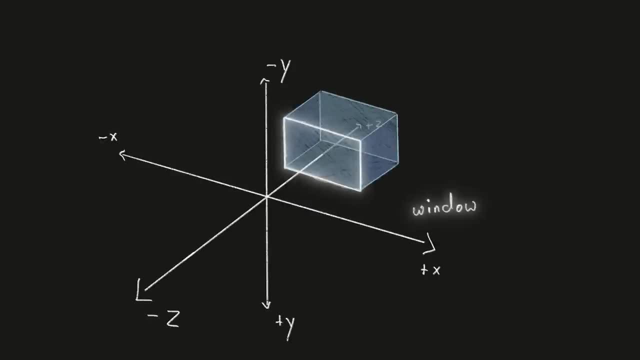 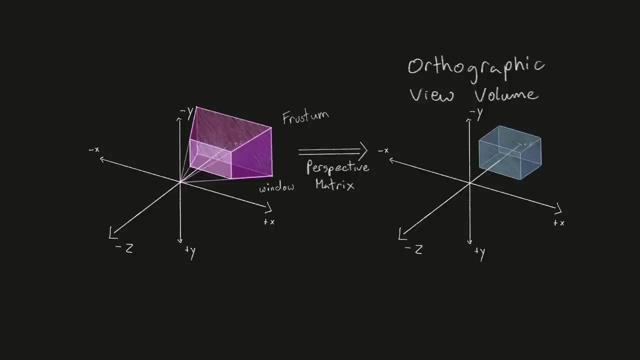 A frustum is the shape that captures a viewer's line of sight, as if they were looking through a rectangular window. So what we want is a perspective matrix that transforms the frustum and any object it can contains into the orthographic view volume. Doing so would apply perspective to all objects within this space. 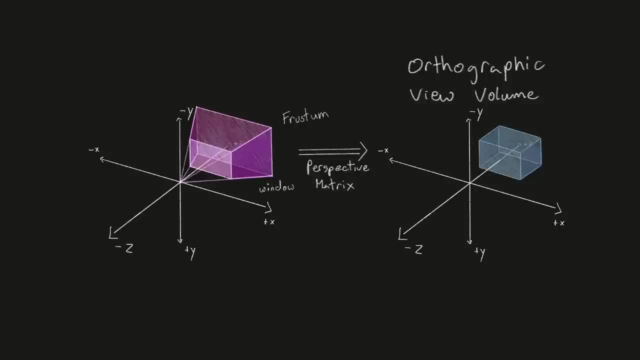 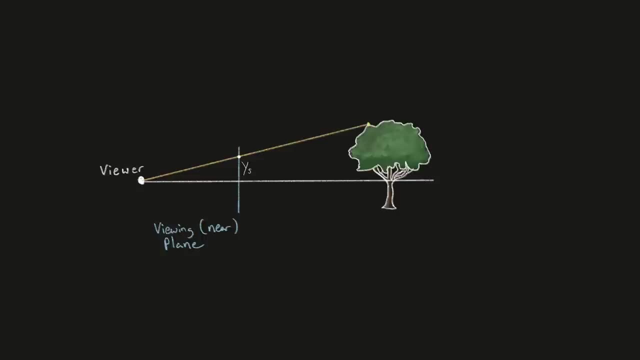 The farther away an object is, the smaller it will appear. To properly apply perspective, we need to project each point onto the viewing plane. For example, to calculate the apparent height of an object on the screen, we can use the property that the side lengths of two similar triangles are proportional to. 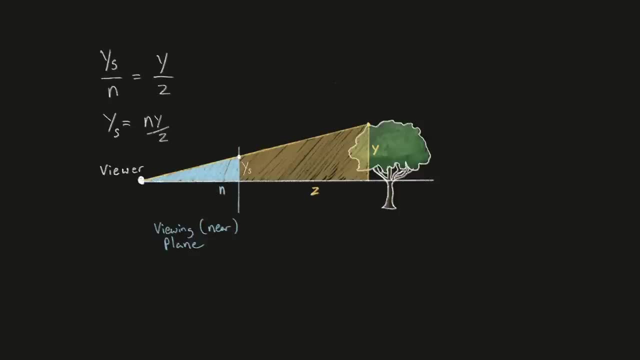 each other. We can rearrange this equation to show that an object's apparent height on screen is equal to the distance to the screen over the distance to the object multiplied by the object's true height. This equally applies for the x direction when calculating an object's apparent width. 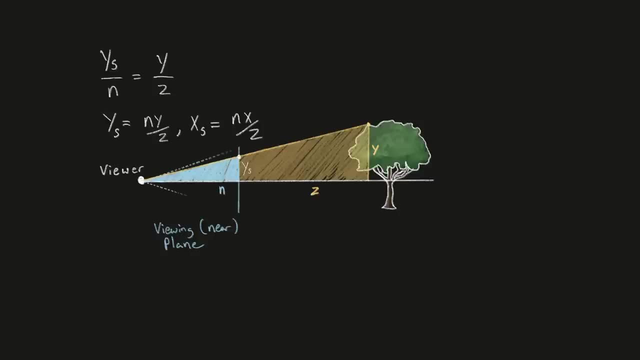 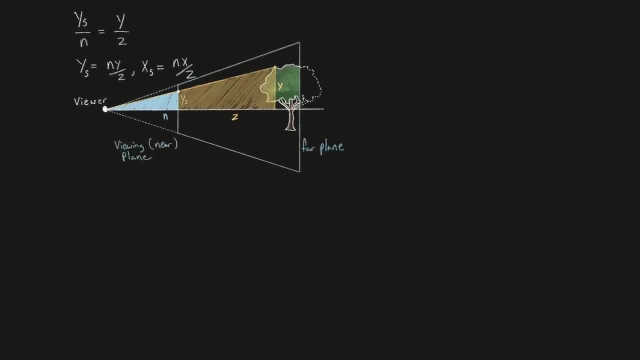 on the screen. Also note that, just as with the other viewing volumes, anything outside of the frustum will be clipped. OK, So what we would like to do is come up with some 4x4 matrix that, when applied to a position vector, 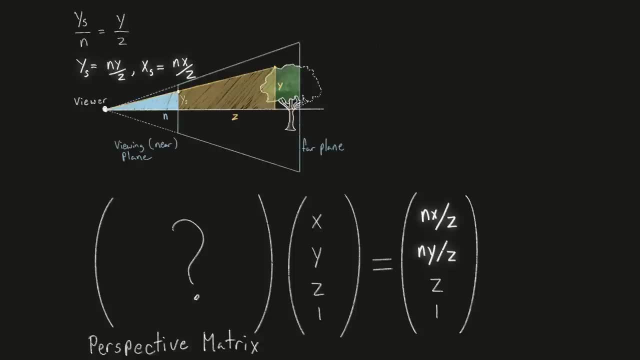 the resulting X gives a maximumچ and y values equal. the projected xs and ys coordinates on the viewing plane. But there is a problem. We have a division by the z component in the solution's x and y components and a 4x4 matrix that can move a z value from here to a division here simply does not exist. 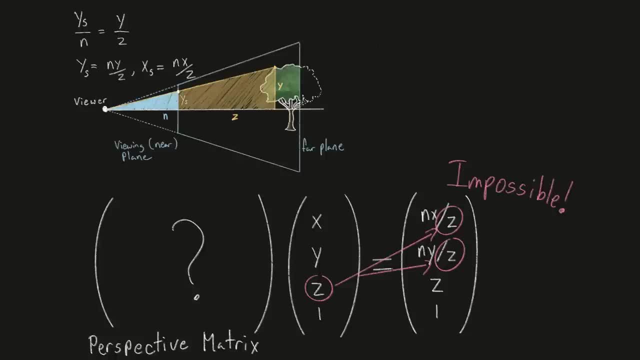 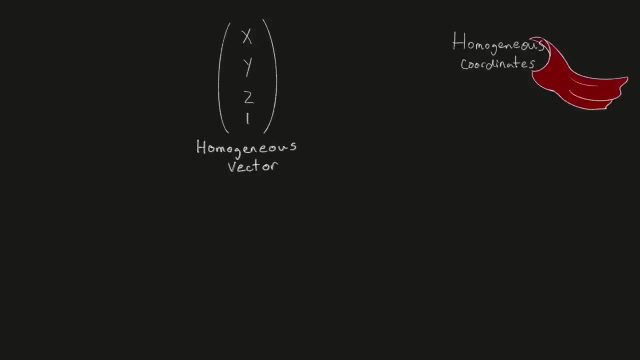 It is just not possible with matrix multiplication alone. But what's that? It's homogeneous coordinates. to the rescue. We have one more trick up our sleeve. So far, the fourth component of all position vectors has been fixed with w always equal to 1. This allows for matrix multiplication. 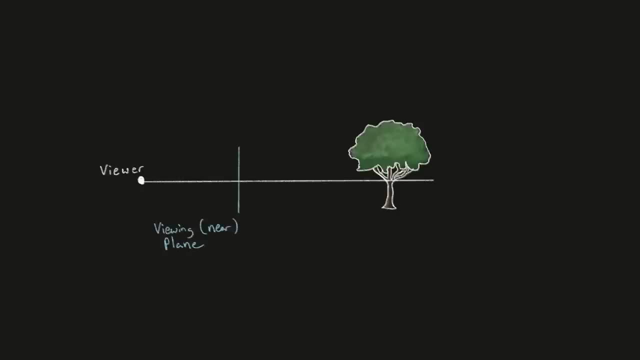 To properly apply perspective, we need to project each point onto the viewing plane. For example, to calculate the apparent height of an object on the screen, we can use the property that the side lengths of two similar triangles are proportional to each other. We can rearrange this equation to show that an object's apparent height on screen 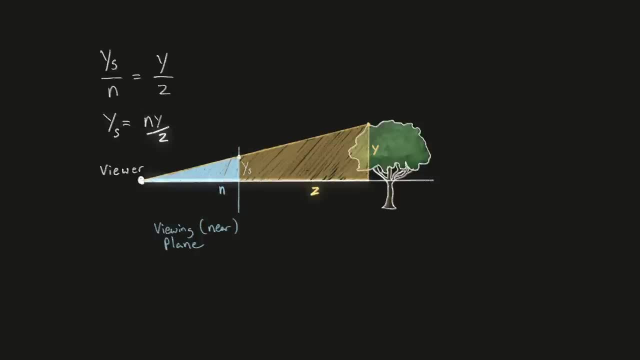 is equal to the distance to the screen over the distance to the object multiplied by the object's true height. This equally applies for the x-direction when calculating an object's apparent width on the screen. Also note that, just as with the other viewing volumes, anything outside of the 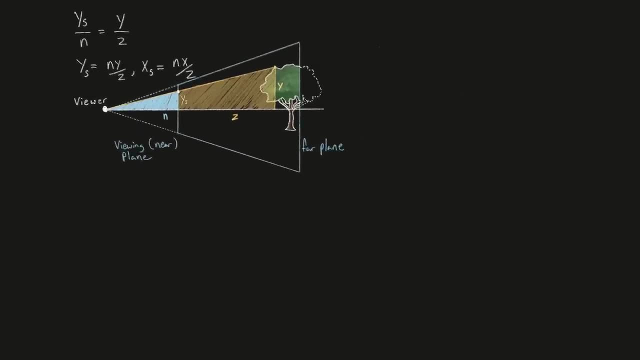 frustum will be clipped. Okay, so what we would like to do is come up with some 4x4 matrix that, when applied to a position vector, the resulting x and y values equal the projected xs and ys coordinates on the viewing plane. But there is a problem. We have a division by the z component. 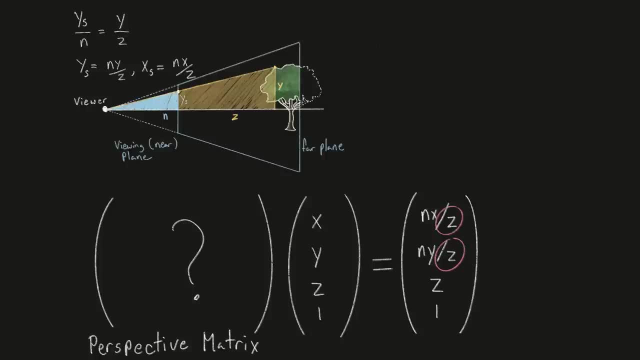 in the solution's x and y components, and a 4x4 matrix that can move a z value from here to a division here simply does not exist. It is just not possible with matrix multiplication alone. But what's that? It's homogeneous coordinates. to the rescue. We have one more trick up our sleeve. 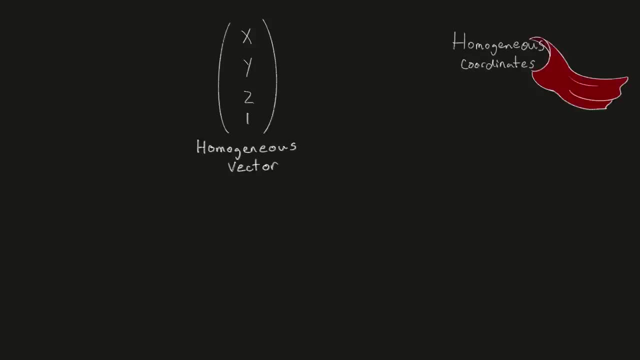 So far, the fourth component of all position vectors has been fixed with w always equal to 1.. This allows for matrix multiplication To implement translations. we will now additionally define w to be the denominator of the x, y and z components. This means that the homogeneous vector x, y, z, w corresponds to the 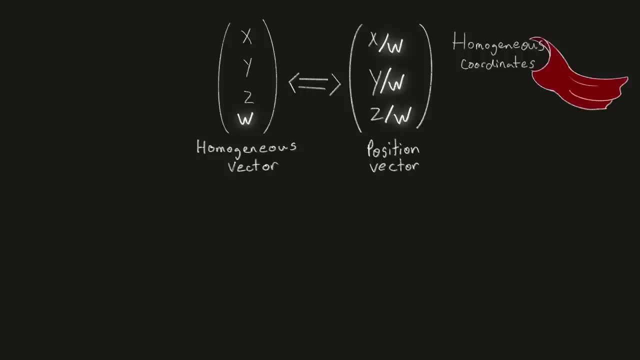 point at x over w, y over w and z over w. This also means that vector 1, 2, 3, 1 is equal to the vector 10, 20, 30, 10, which is also equal to the vector 2, 4, 6, 2.. These all represent the exact same. 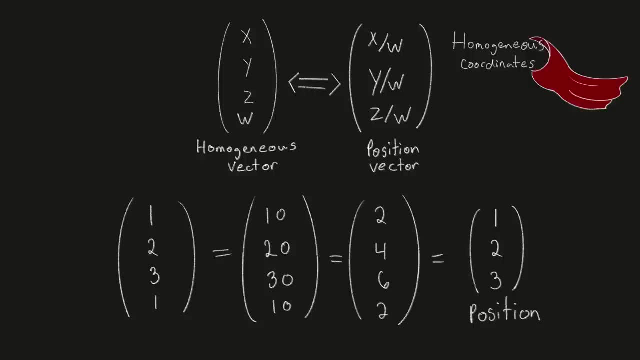 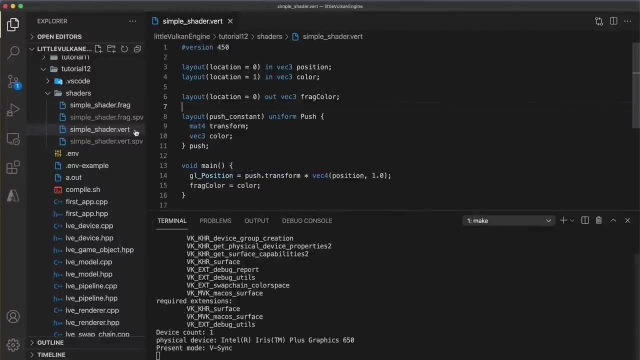 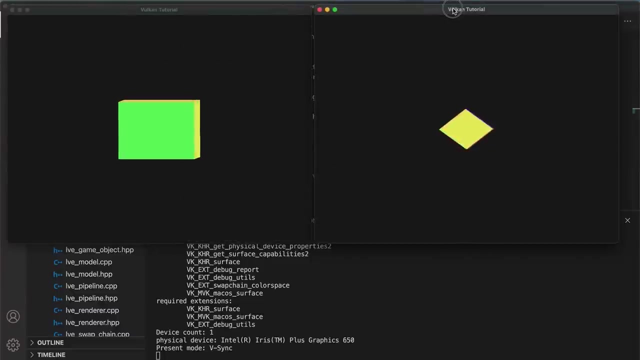 at This. division by w is automatically applied on the GLPosition variable output from the vertex shader and has always been occurring. If I go into our vertex shader and update the homogeneous coordinate value to 2 and run my code, my object becomes half the size because we now divide each position component by two. Therefore, 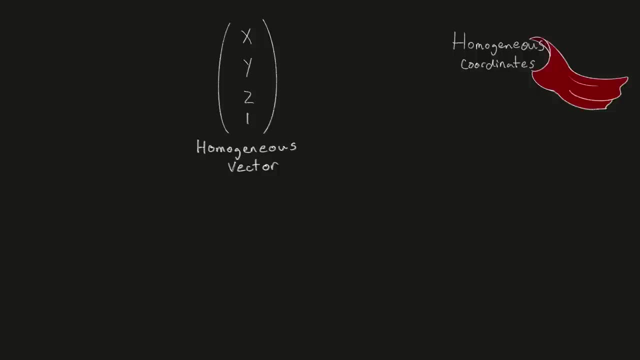 to implement translations, We will now additionally define w to be the denominator of the x, y and z components. This means that the homogeneous vector x, y, z, w corresponds to the point at x over w, y over w and z over w. 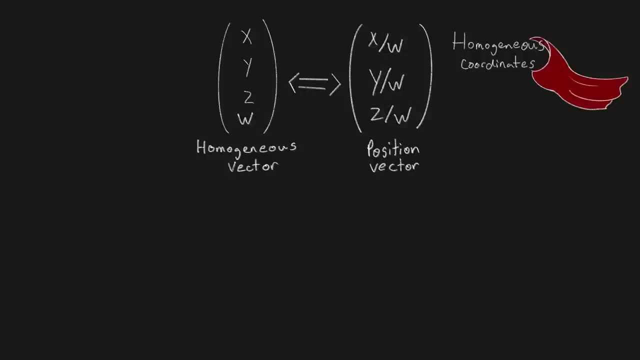 This also means that vector is equal to the vector, which is also equal to the vector. These all represent the exact same position. at This, division by w is automatically applied on the glPosition variable output from the vertex shader and has always been occurring. 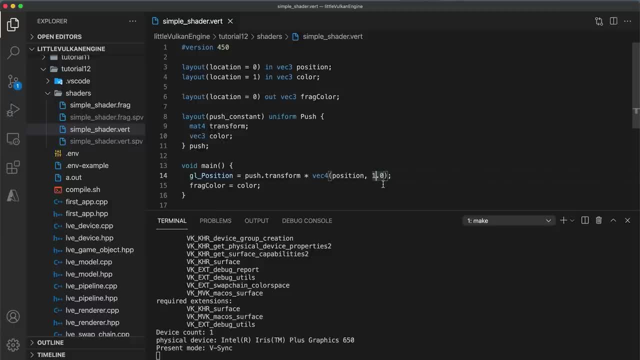 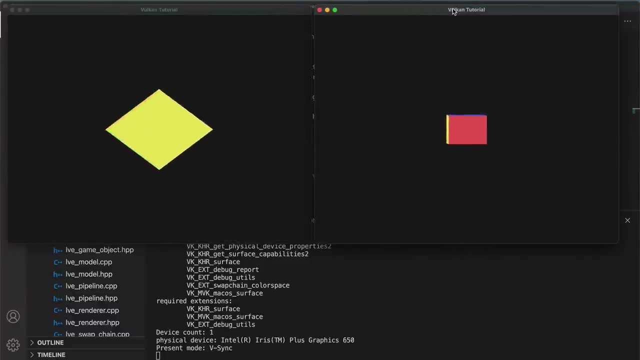 If I go into our vertex shader and update the homogeneous coordinate value to 2 and run my code, my object becomes half the size because we now divide each position component by 2.. Therefore, if the solution's w component is equal to z, it will be possible to calculate. 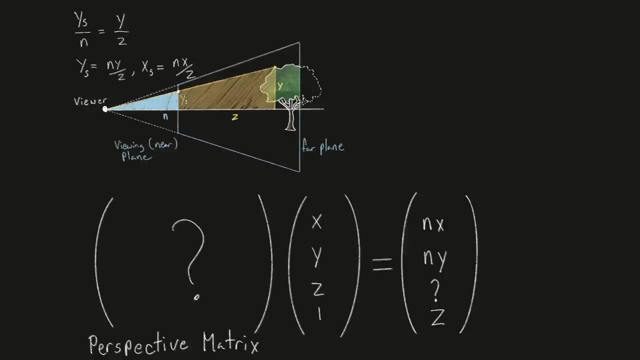 the projected coordinates of x and y onto the viewing plane. With this knowledge we can start to construct the perspective matrix transformation. The first two rows have the distance to the viewing plane on the main diagonal and zeros elsewhere. This will have the effect of: 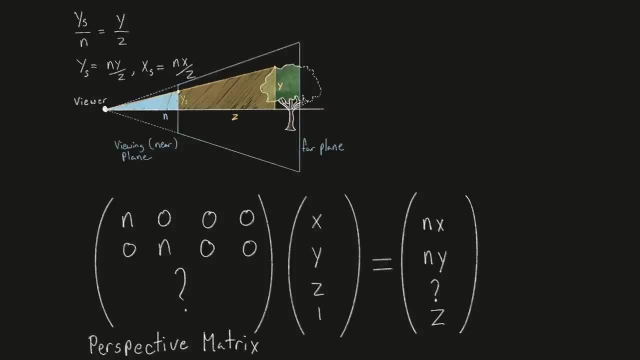 dividing the two components by the distance to the near plane. Next, the final row must be to take the z component from the input vector and move it to the w component of the solution vector. Now all that's remaining is the third row, and an easy mistake to make is to think this: 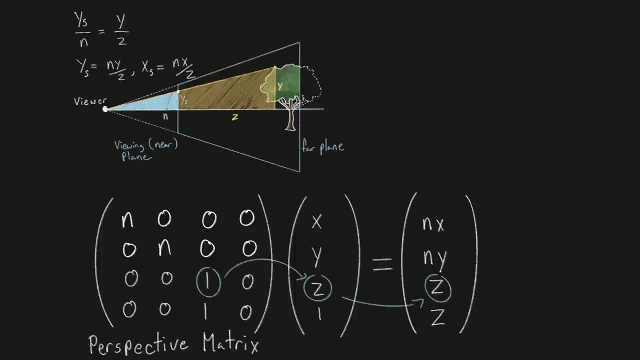 can also just be to copy the z depth values into the solution. The problem is, every component will be divided by w, so we'll just have to do the same thing with the z component. So we're done with this. one z over z is just 1, and now we've lost our depth information. 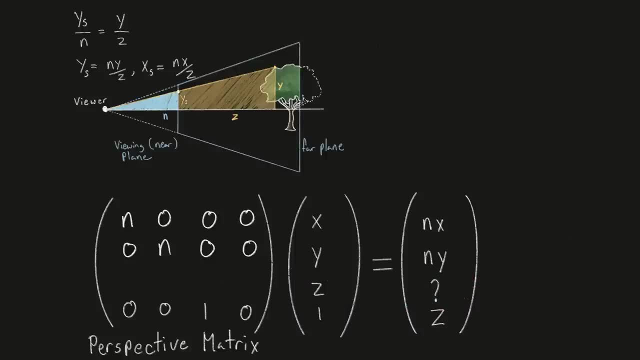 and won't know which objects should be drawn in front of the others. So rewind, and in reality we need the solution's z component to equal z squared, since z squared over z is equal to z, but in our matrix we only have two remaining unknown values to use If we multiply this out. 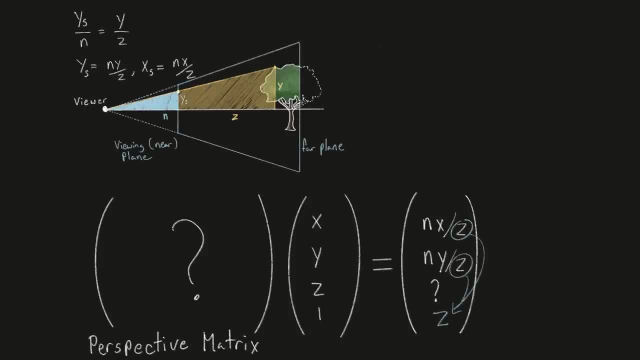 if the solution's w component is equal to z, it will be possible to calculate the projected coordinates of x, z and y. transform only by a half the squareический quadrant value from the vertex shader and the double squarecificfecture component of the solution's 3,2 to perfect quadratic. That is how v and w are coded by abtion at. 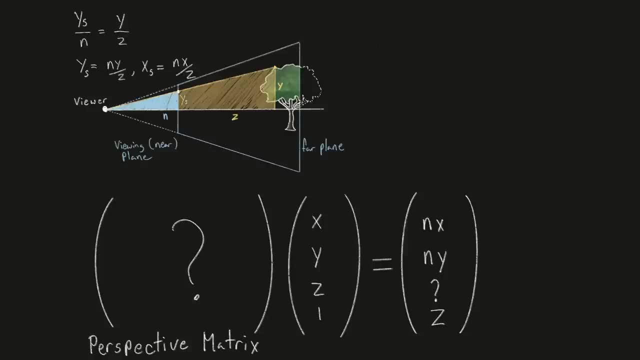 here we already learned some techniques we are still looking for, and that is where these leftovers are located, By solving the thank. outside of these developments, I am now of x and y onto the viewing plane. With this knowledge we can start to construct the perspective matrix transformation. The first two rows have the distance to the viewing plane on. 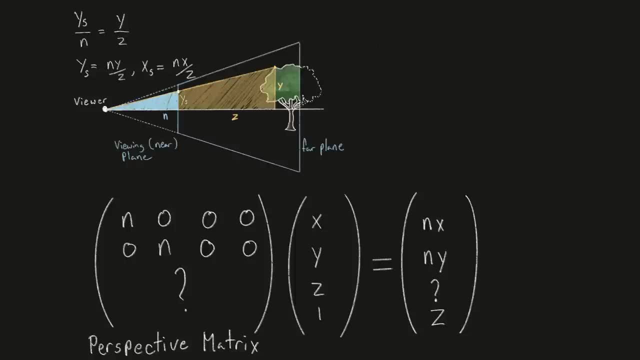 the main diagonal and zeros elsewhere. This will have the effect of scaling the x and y components by the distance to the near plane. Next, the final row must be to take the z component from the input vector and move it to the w component of the solution vector. 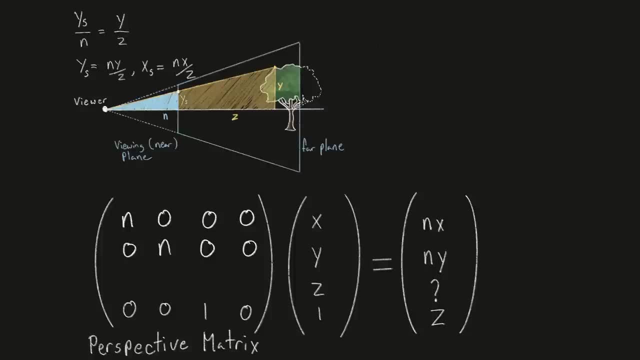 Now all that's remaining is the third row, and an easy mistake to make is to think this can also just be 0, 0, 1, 0. to copy the z depth values into the solution. The problem is, every component will be divided by w, including this one. z over z is just 1, and now we've lost. 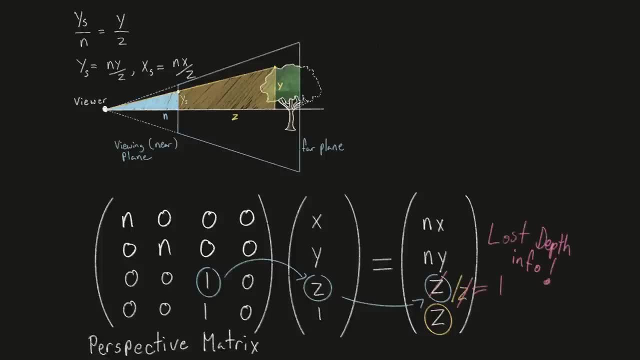 our depth information and won't know which objects should be drawn in front of the others. So rewind, and in reality we need the solution z component to equal z squared, since z squared over z is equal to z, but in our matrix we only have two remaining unknown values to use. 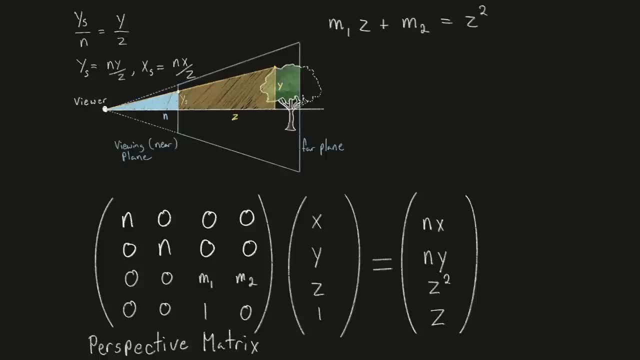 If we multiply this out, we get the equation: m1 times z plus m2 equals z squared. This is a quadratic equation, meaning it has at most two real solutions and can't be true for other z values, values. Therefore, we will add two constraints: that this equation is only true when z equals. 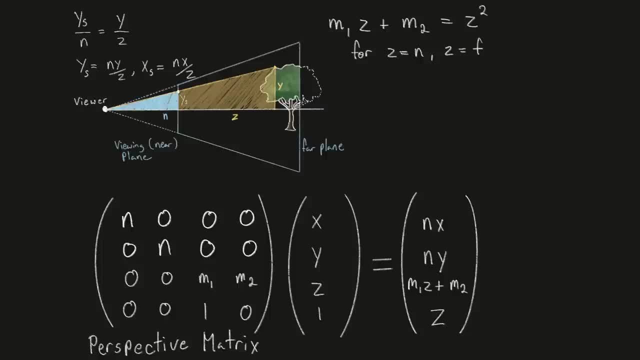 n or z equals f. This means that the transformation will not change the z values for points on the near and far planes, but all other z values will be warped non-linearly. This results in two equations that we can use to solve for m1 and m2.. m1 times n plus. 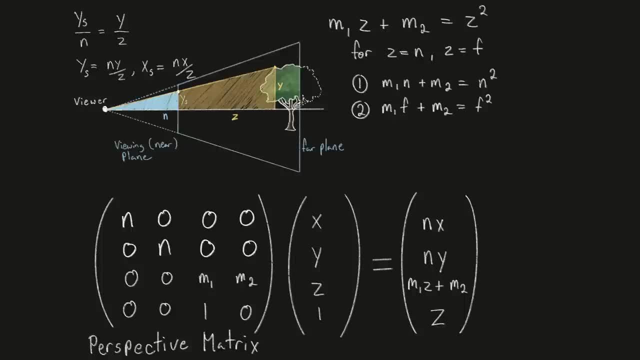 m2 equals n squared and m1 times f plus m2 equals f squared. Solving these equations, we get: m1 is equal to f plus n and m2 is equal to negative f times n. Let's plug this in and the solution z component becomes f plus n times z minus fn. 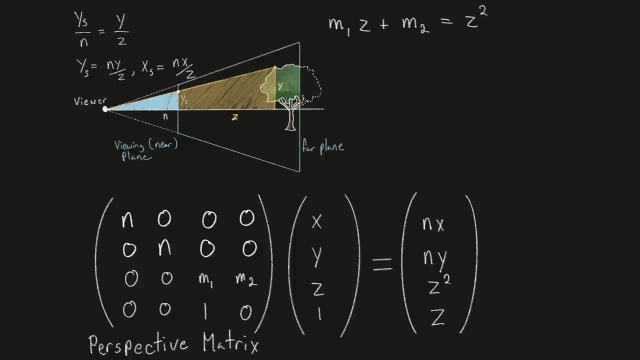 we get z squared. This is a quadratic equation, meaning it has at most two real solutions and can't be true for other z values. Therefore, we will add two constraints: that this equation is only true when z equals n or z equals f. This means that the transformation 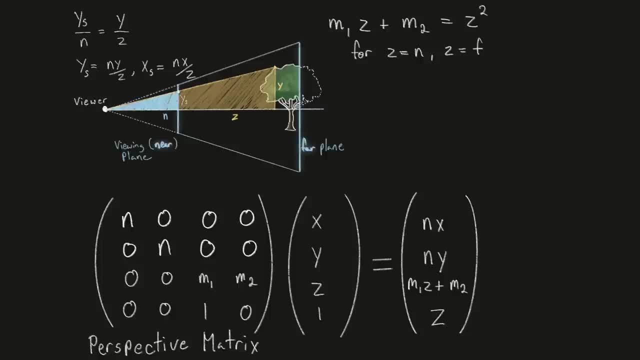 will not change the z values for points on the near and far planes, but all other z values will be warped non-linearly. This results in two equations that we can use to solve for m1, and m2.. m1 times n plus m2 equals n squared, and m1 times f plus m2 equals f squared. 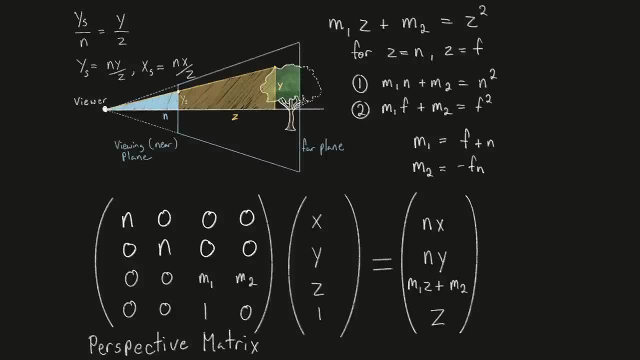 Solving these equations, we get: m1 is equal to f plus n and m2 is equal to negative f times n. Let's plug this in and the solution z component becomes f plus n times z minus fn. So let's take a minute to go over what this really means. 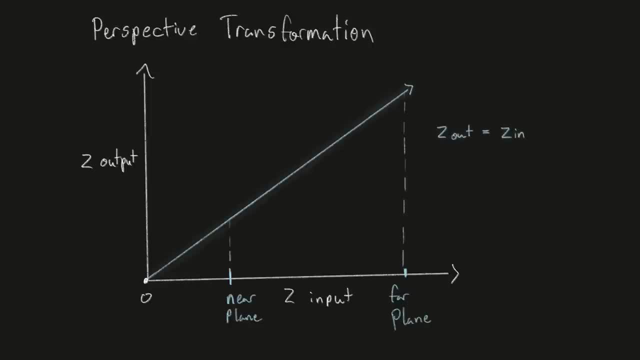 We wanted to have a one-to-one linear relationship between the input z value and the output z value, But the best we could do is make this true for points at the near depth and far depth planes. The z depth values on the near and far planes remain unchanged, but the relationship is no. 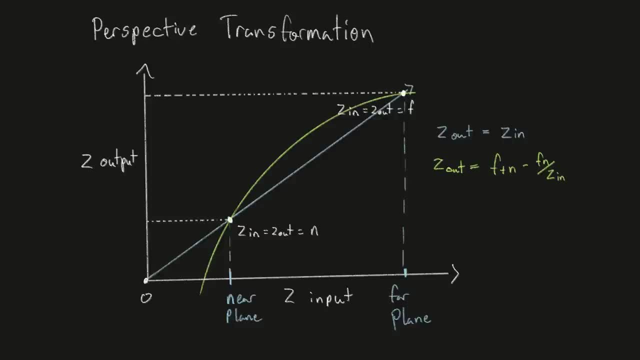 longer linear. However, this is still useful because the relative ordering of the z values between the near and far planes is preserved. This means we can still use z to determine the ordering of objects within our scene, An advantage to having the z depth values be non-linear. 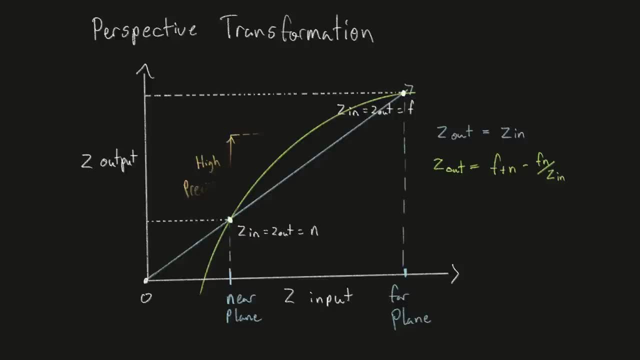 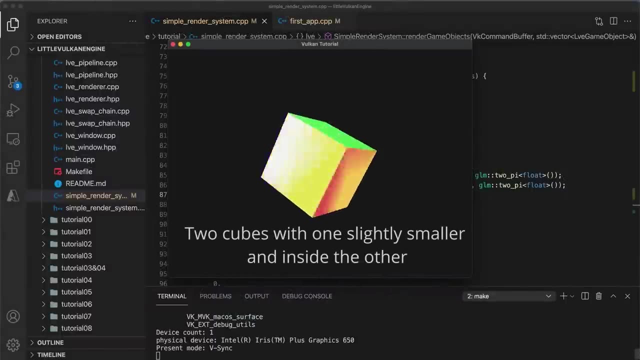 is that calculations, that they do not have to be non-linear, and that they can be non-linear is that the near plane will be higher precision than calculations at the far plane, reducing observable z-fighting. Z-fighting also known as stitching or depth fighting. 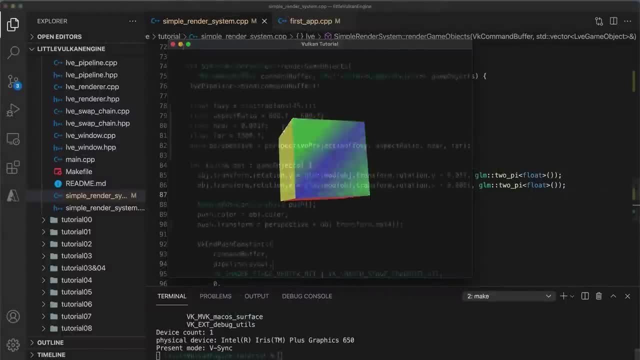 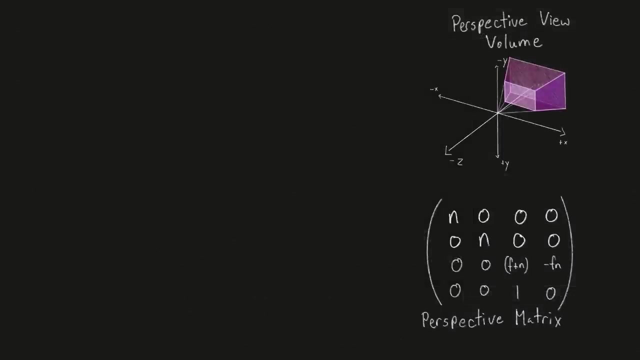 occurs when two surfaces are very close together. This visual artifact is caused by the rounding errors of floating point calculations and can be avoided by reducing the distance between the near and far planes. Now back to the perspective matrix. If you apply the perspective transform, 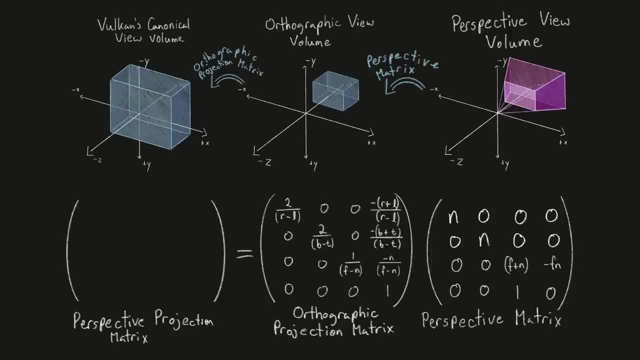 followed by the orthographic projection transform. the combined result is known as the perspective projection transformation, And this is what we've been after. This matrix will transform objects contained by the viewing frustum into the canonical view volume and, in doing so, will make the objects appear in perspective. We define the perspective projection. 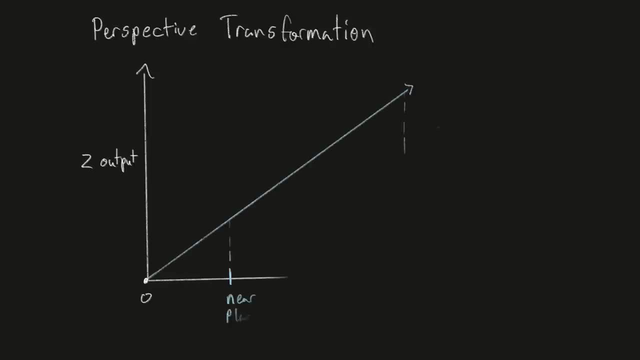 So let's take a minute to go over what this really means. We wanted to have a one-to-one linear relationship between the input z value and the output z value, but the best we could do is make this true for points at the near depth and far depth planes. The z depth values on the near 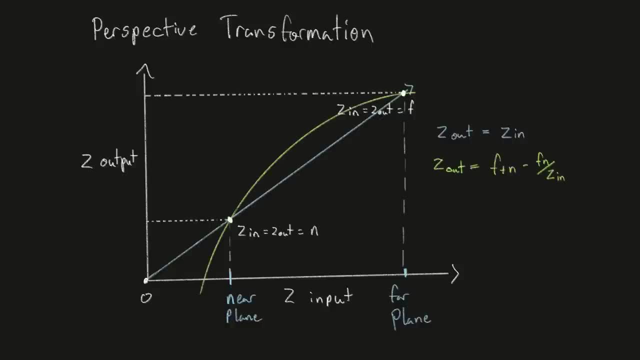 and far planes remain unchanged, but the relationship is no longer linear. However, this is still useful because the relative ordering of the z values between the near and far planes is preserved. This means we can still use z to determine the ordering of objects within our 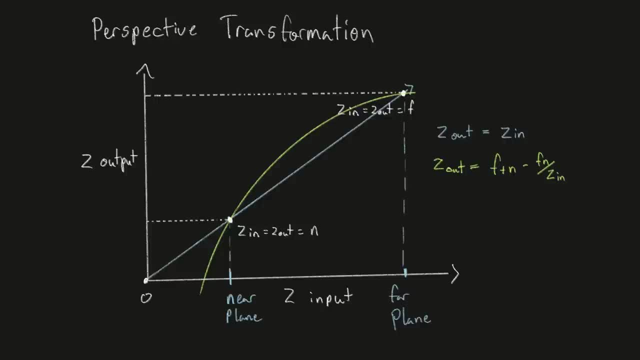 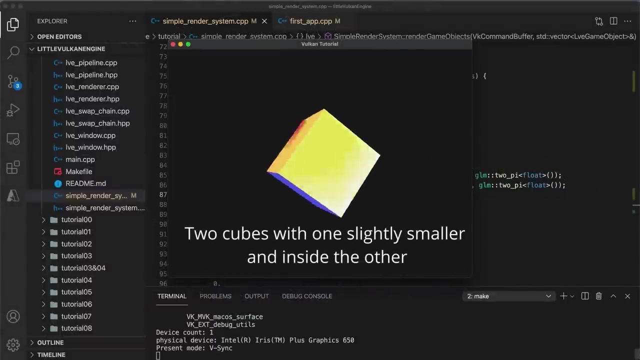 scene. An advantage to having the z depth values be non-linear is that calculations at the near plane will be higher precision than calculations at the far plane, reducing observable z-fighting. Z-fighting, also known as stitching or depth-fighting, occurs when two surfaces are very close together. This 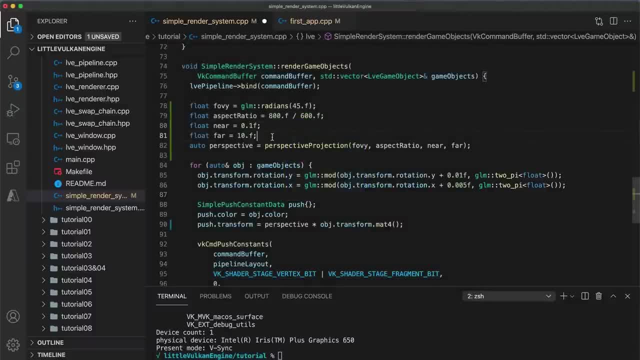 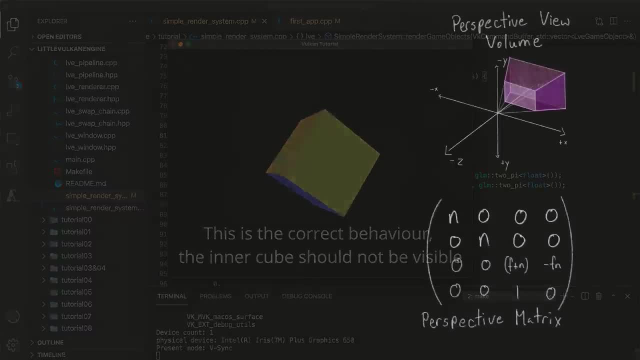 visual artifact is caused by the rounding errors of floating point calculations and can be avoided by reducing the distance between the near and far planes. Now back to the perspective matrix. If you apply the perspective transform followed by the orthographic projection transform, we get the following: 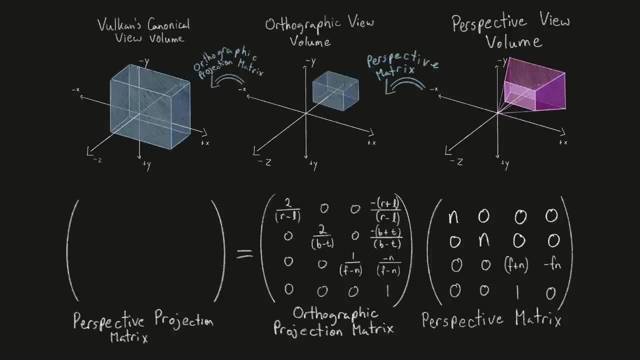 The perspective transform is the perspective transform, followed by the orthographic projection transform, followed by the perspective transform, followed by the orthographic projection transform. then the combined result is known as the perspective projection transformation, And this is what we've been after. This matrix will transform objects contained by the viewing. 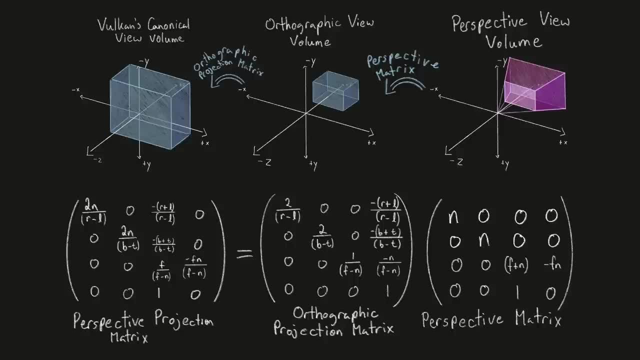 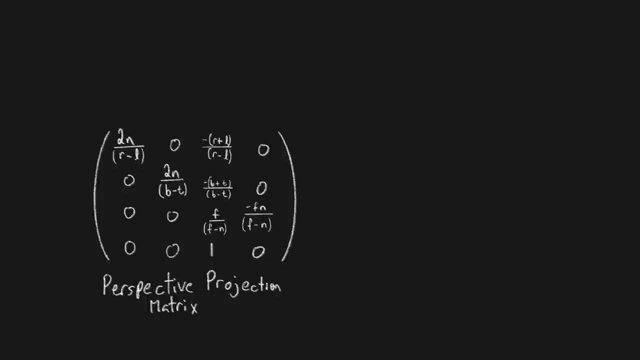 frustum into the canonical view volume and in doing so will make the objects appear in perspective. We define the perspective projection matrix with the same values as used by the orthographic view volume, the six values r, l, b, t, n and f, but it's often more convenient. 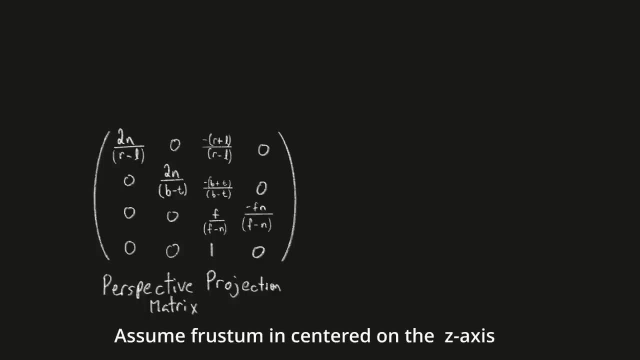 a simpler system where we assume the frustum is aligned along the z-axis, meaning that we are looking through the center of the window. This implies that left is equal to negative right and top is equal to negative bottom, which then can be used to further simplify the matrix. 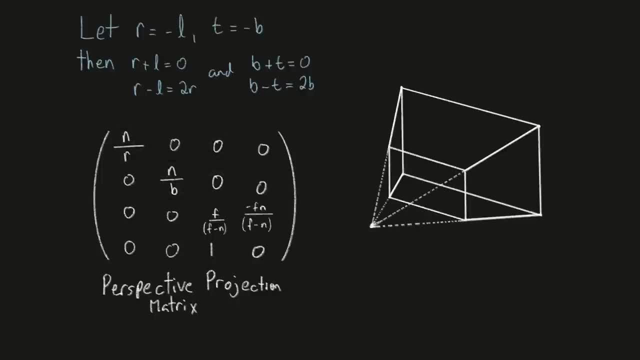 Finally, it is common to specify a vertical field of view rather than use the values for the bottom and the right planes. The vertical field of view is the angle from the bottom to the top of the near plane relative to the viewer's line of sight. If we also know the